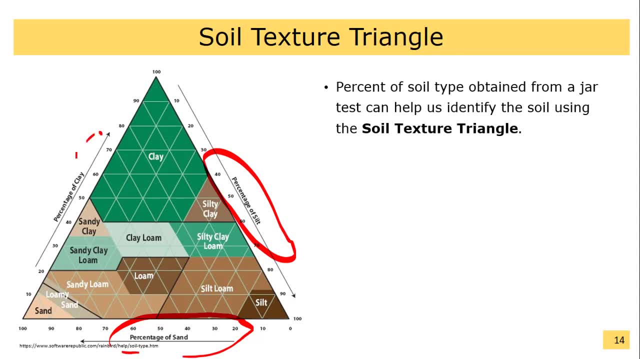 on the third axis you have percentage of clay. The soil texture triangle was developed by the United States Department of Agriculture, USDA. Using it, you can classify the soil into 12 different types, such as clay loam or sandy loam, et cetera. 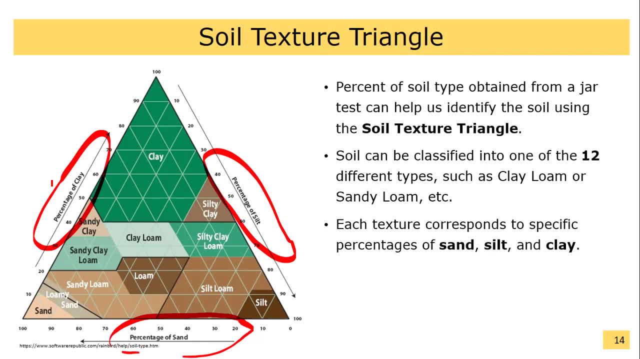 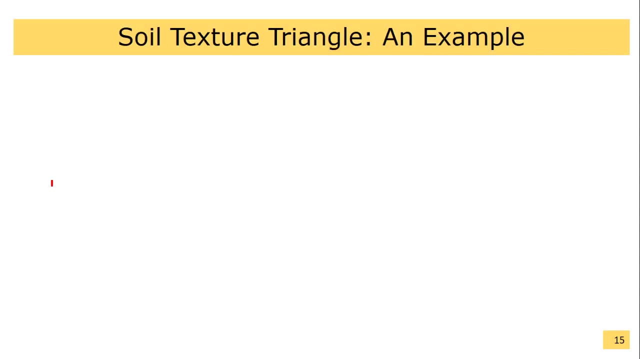 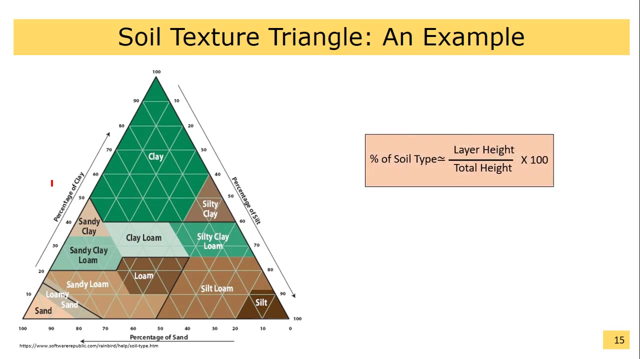 Knowing the texture of your soil helps you manage it and modify or condition it if necessary. Soil texture triangle- an example. Let's now see an example of how we can make use of the soil texture triangle to identify the soil type iques on your permaculture plot, based on the formula shown on this slide we have. 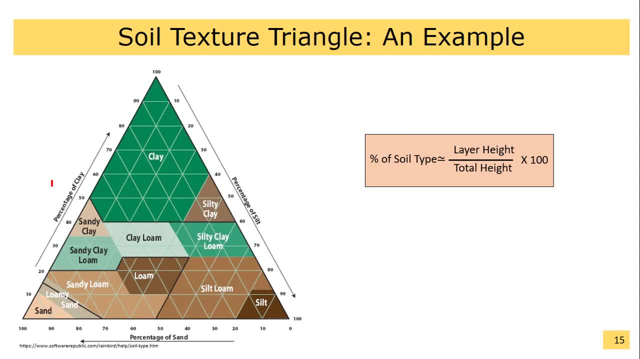 arrived at the percentage of sand, silt and clay for our soil, as shown in this table. now we can see where these percentage plot on the soil texture triangle: 10% sand is here. 60% silt is there. 30% clay is there, based on the 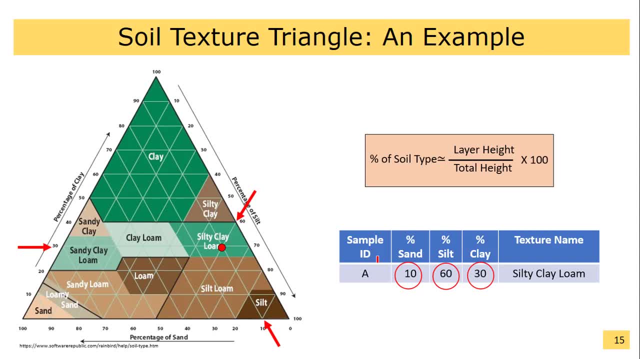 results of the Tsar test, our soil plots in the area labeled silt and clay: clay loam. As you can see, it is quite straightforward to make use of the soil texture triangle once you have results from a jar test. One thing you should keep in mind: that jar test must be conducted on soils taken from many 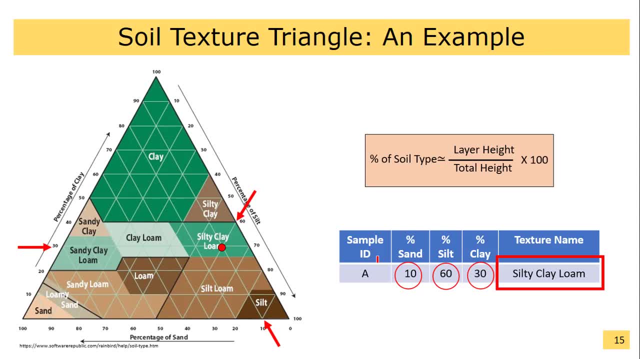 different sites on your plot and the results averaged. If you take soil from only one location, we may get a biased result.